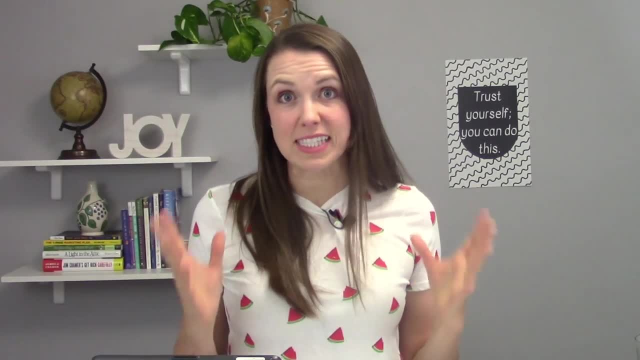 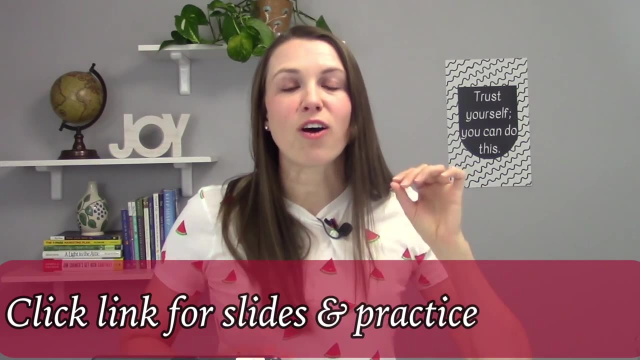 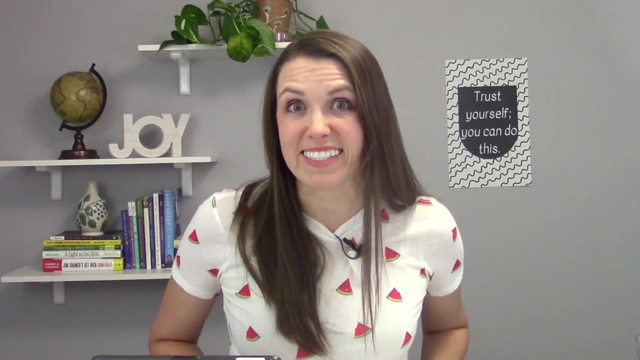 of thing. But I do also have these slides that I'm using available for you to download with the, and so click the link down below. and I also have extra problems, because the best way to learn something is to practice it over and over, right? okay, let's get. 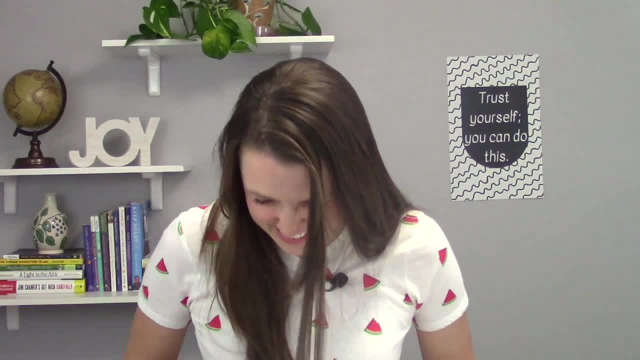 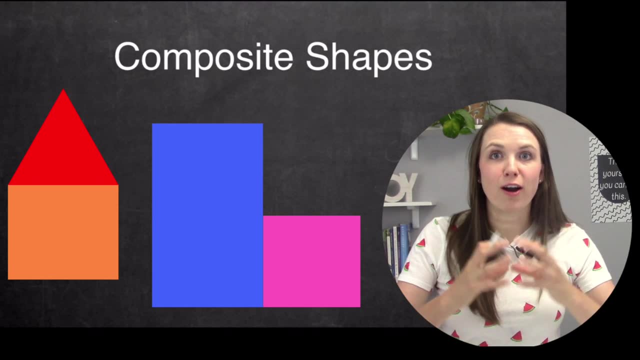 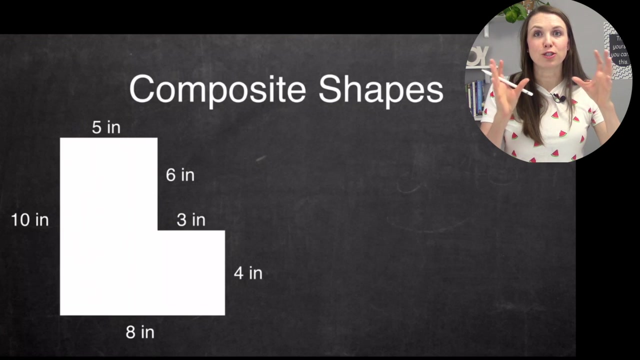 started on compositing some shapes. so, as I mentioned at the beginning of the video, a composite shape is really just two shapes that are combined together. so what you want to do first is you want to dissect your shape, your miss shaped shape, and, if you can divide it into two different shapes and find the area of 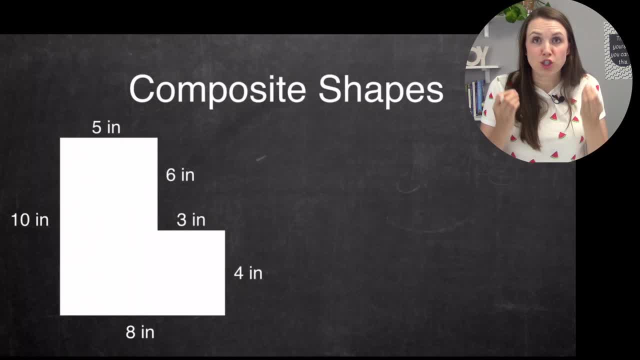 those two different shapes. it will make your life so much easier. and I also like to kind of think about: well, what is this? so I look at this shape and I think of it is a pan of brownies and somebody ate some. so if you're like me, you kind of like to even it out, right? so 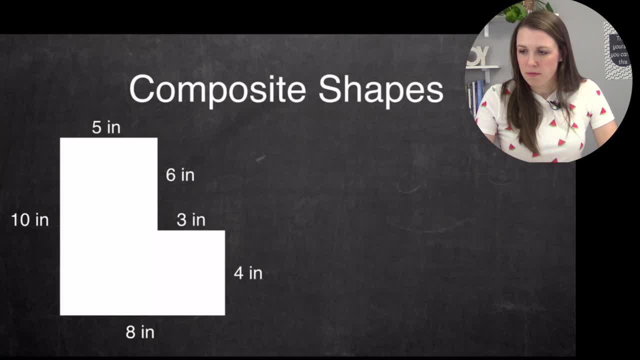 we're gonna even it out, ok, so we're going to even it out right here. so now our plate of brownies is full, like that, ok? so I essentially have two different shapes: I have this long rectangle and then I also have this shorter rectangle. so if you remember the way to figure out, 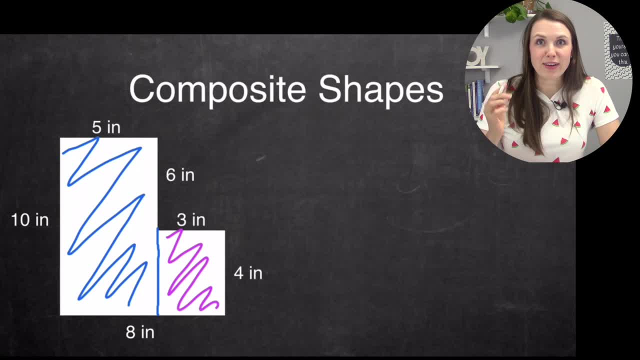 a shape. shape, or at least a rectangle, is basically length times width. okay so, length times width, okay. so let's take a look at this blue guy right here. so my length here is 10, so I'm going to go 10 times my width and my width here is 5. so 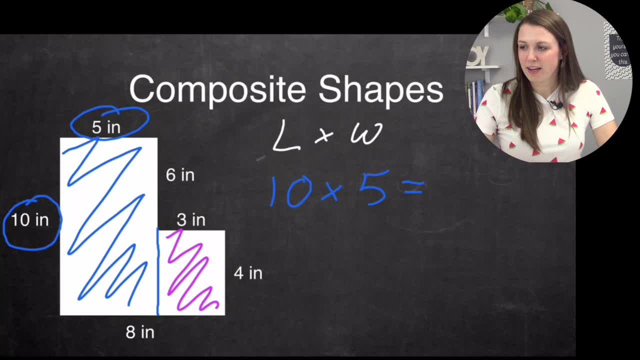 I have 10 times 5, and what is 10 times 5? 50, right? okay, and now I have my smaller rectangle. my length is 3 and my width is simply 4, so 3 times 4 is 12, and then I have just I add them together and 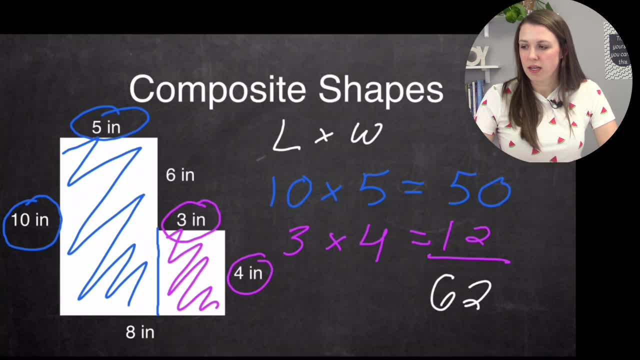 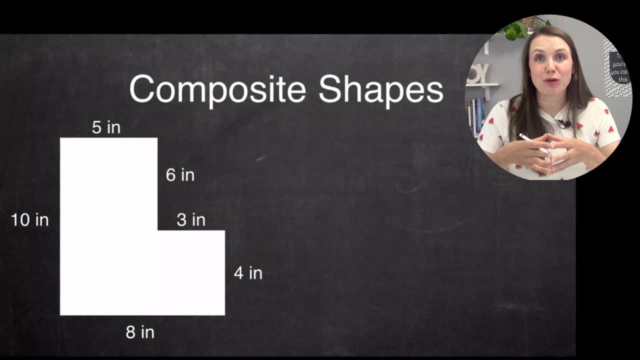 50 plus 12 is 62 inches squared, and so that is going to be my answer. now, the way that I just showed you is one way to do it. however, you don't have to slice your brownies that way. you can slice your brownies the other way as well, so. 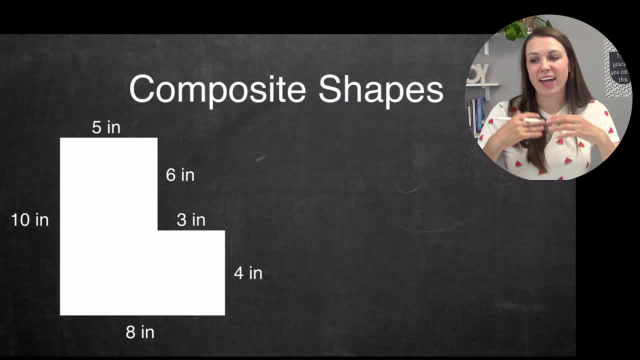 I'm going to show you the same problem and we're going to try it just a different way. so again, I want to make sure that I do length times width, length times width, length times width. so this time I'm going to cut it right here and I have this little area right. 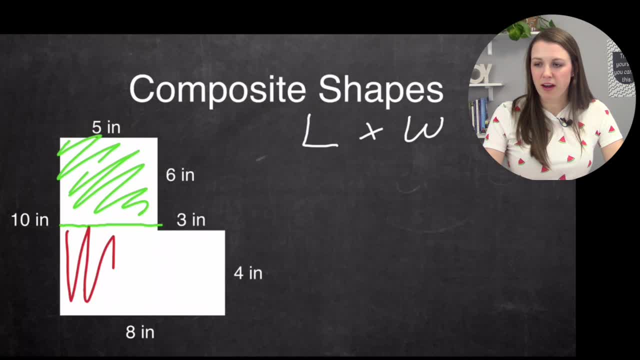 here, and then I have this area right here. red and green must be Christmas colors, right? okay? so length, times, width, and you want to really make sure that you're looking at the correct numbers. so if you look here at this 10 inch- well, if I use that, oh my goodness, that goes like: 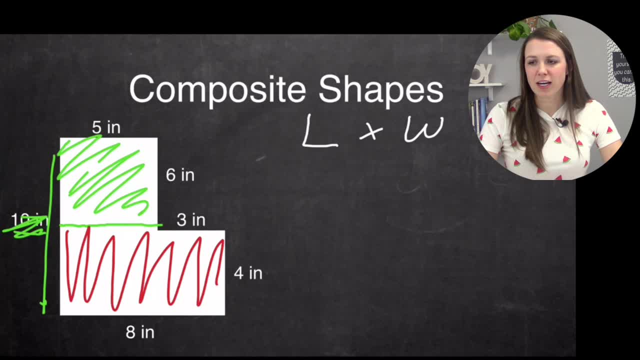 all the way down. right, that's not what I want, so here I'm going to use my 5 inch and my 6 inch. so I have here: the length is 5 times the width. I actually am doing it backwards, but it's fine. so 5 times 6 is simply 30. right, and now we? 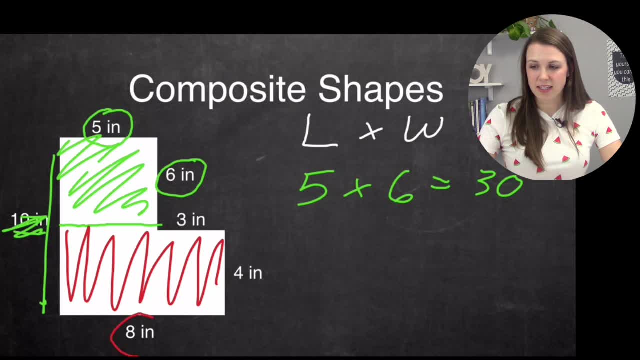 have our red and so I have a no matter of color. so the number of times I'm just going to add this is 8x4, and so again this 3. in this case it doesn't really matter. so you want to make sure that you're looking at the correct numbers, because a lot of times 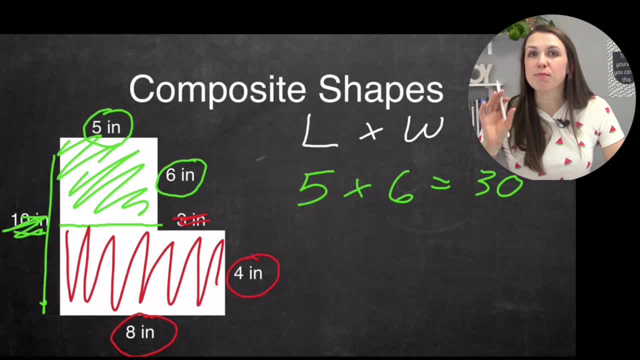 there might be extra numbers that you don't need. sometimes you even actually have to subtract numbers, so just be mindful of that. so 8 x 4 is 32, right, and so if I go 30 plus 5, that's a equal to 8. so 8 x 4 is 32, and that's the number of times we're going to. 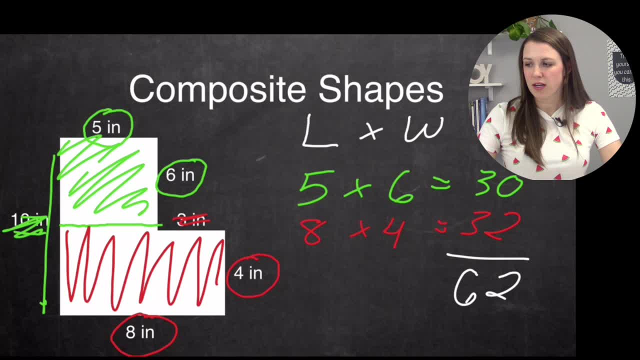 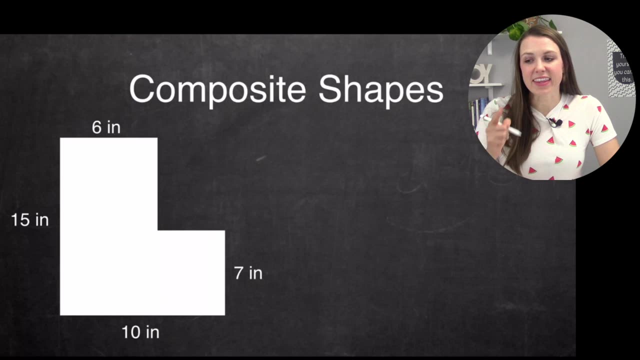 plus 32 is 62 inches squared, And that's what I got before, right? So my answer works the same way, no matter which way I do it. Let's practice another one, okay? So you can see here that this one 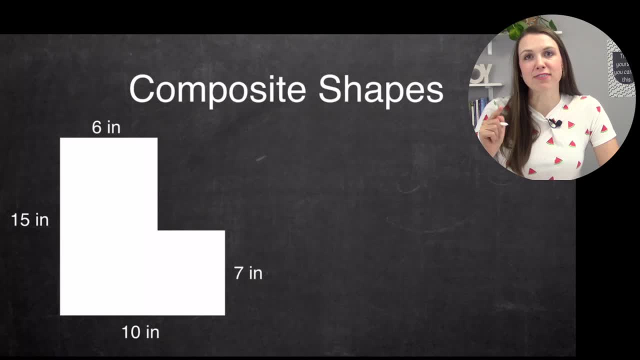 actually doesn't provide me with quite as many numbers, so I might have to actually do just a little bit of math, But first thing we're going to do is we're going to separate it. okay, And I am going to just separate it right here. 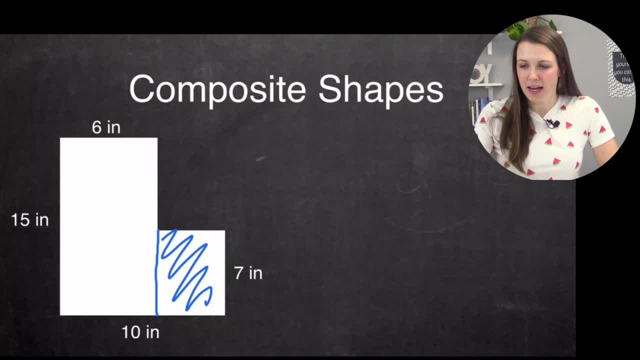 So I have this piece right here, and then I have this piece right here, Okay. so notice, here I have my length times, my width, length times width. Okay so here I have seven inches, so that's sometimes it's also called length times height. 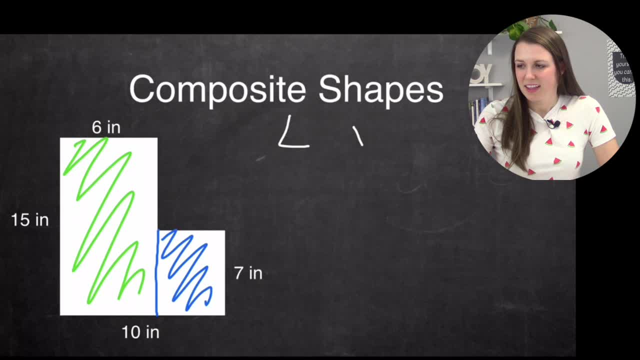 So let's actually call it length times height, this time Length times height. okay, So I have my seven, so that's actually the height, right, But look here at my 10.. So the 10 is actually not it, right. 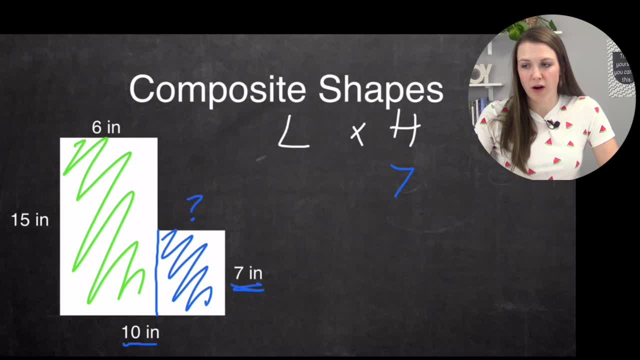 But I don't have it right here. This is really what I'm looking for. So what I'm going to have to do is I'm going to have to go 10 minus this six right here, here, which is four. So if I put four right here- I know this is an arrow, I know that- six plus four. 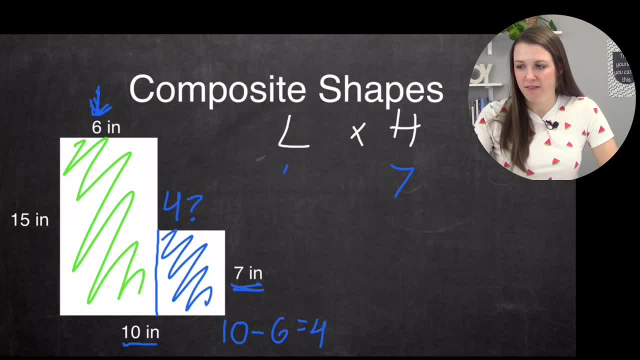 equals 10.. So that's my answer. So I simply have seven times four, which is 28.. And now let's do the green one. Looks like I don't have to do any extra math on the green, So I have my length. 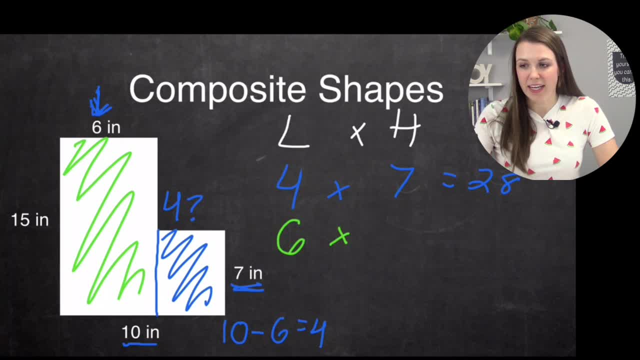 which is six times my height, which is 15.. And I simply get 90.. Add the two together: 28 plus 90. So we have the eight. bring it down: 118 inches squared. So again, you're really going to want to make sure that you click the link down below so that. 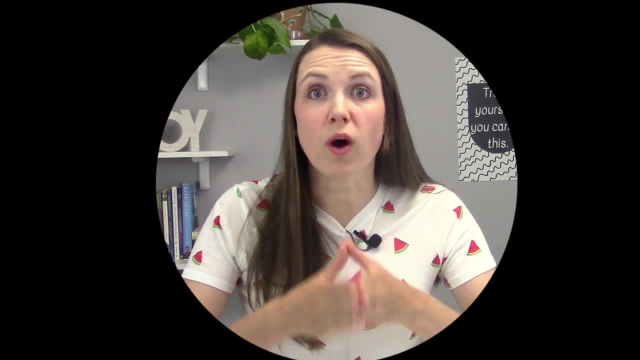 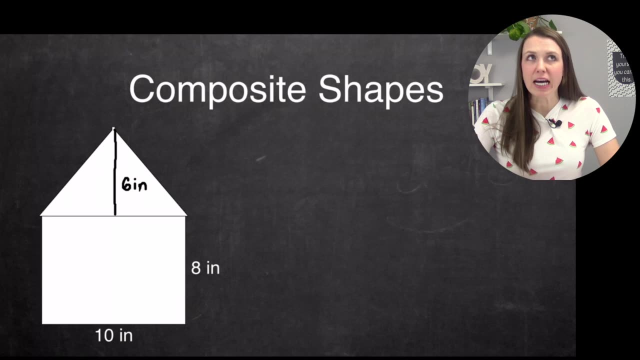 you can gather my slides with the answers and then also do a little bit of extra practice, because it will just help you so much. So now I'm finding the area of either a house or a rocket ship. right, Use your imagination. So we're going to just start with the rectangle that's at the 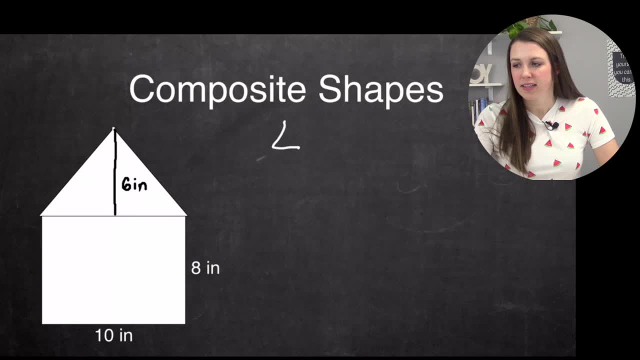 bottom, because we know that that is the length times width. That's how you find the area of a rectangle. Okay, So the rectangle which is the height, which is the width, which is the length. here I have my 10 inches and my 8 inches, or I guess, like I said before, times. 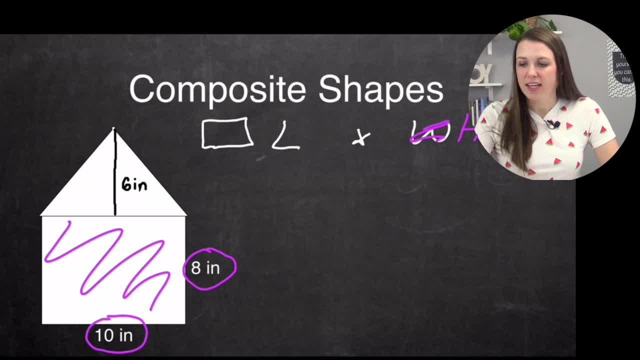 height, length times height, so I have: the length is 10 times the height, which is 8, and that gives me 80. okay, now to find the area of a triangle. it's actually one step more okay, so we're going to make the triangle blue, and so what I'm going? 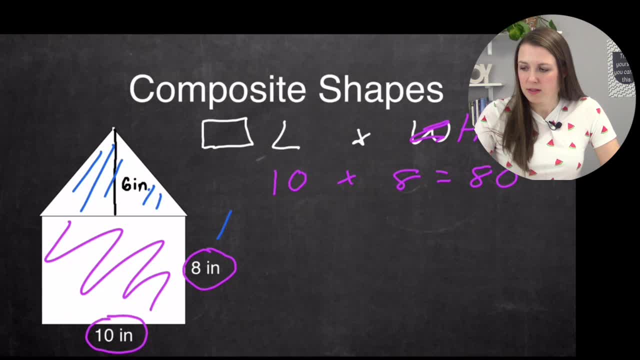 to have to do to find the area of the triangle. let me bring that back to white. the area of a triangle is 1 half based times height. okay, so it's slightly different. so what I'm going to do is I need to bring down that 1 half and my 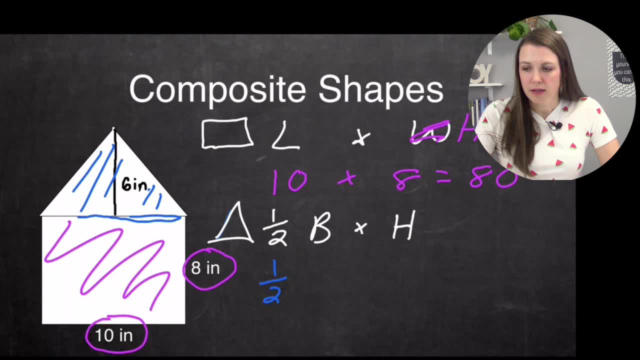 base is right here. but notice, that's that 10, right? so I'm going to put that 10 against. we have 1 half base, so 1 half times 10 times my height, and my height is that 6 inches. so what is 1 half of 10? that's simply 5, right? and then bring down my 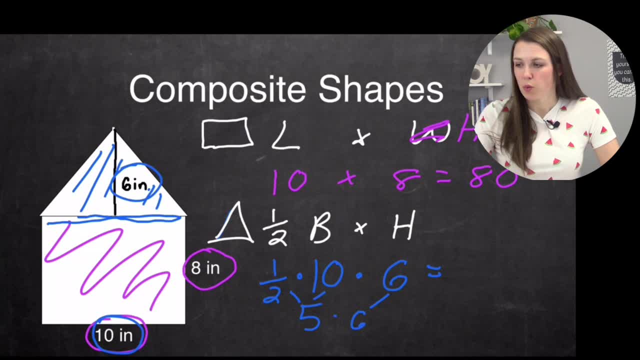 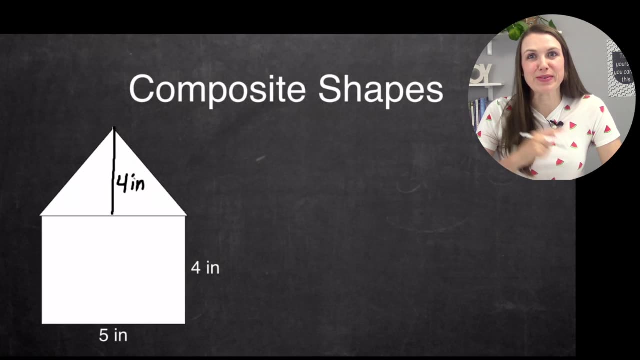 6 and I have 5 times 6, which is 30. add the 2 together and the square root of 6, 80 plus 30, is going to be 110 inches squared. Another practice with our house or our rocket ship. So I'm going to start off with my rectangle at the bottom, So we have area of the rectangle. 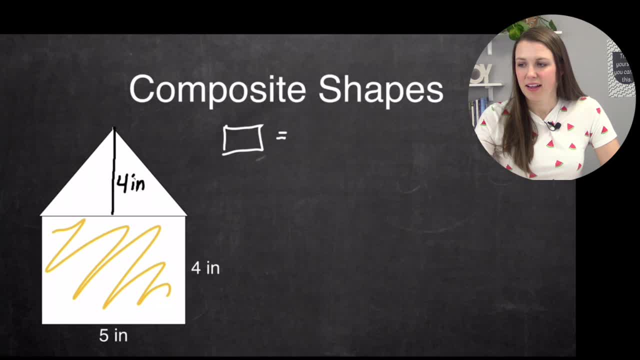 equals length times height. So I have simply five times four, which equals 20.. And now I have my little top part. So to find my triangle, it is going to be one half base times height equals length times height. So I'm going to start off with my triangle at the bottom.